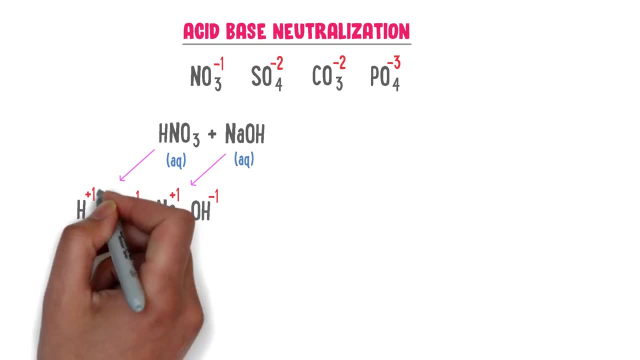 into sodium ion and hydroxide ion. Now the positive part of acid reacts with the negative part of base and the negative part of acid reacts with the positive part of base. I mean hydrogen ion react with hydrogen ion and nitric ion, Hydroxide ion to form water and nitrate ion react with sodium ion to form aqueous solution. 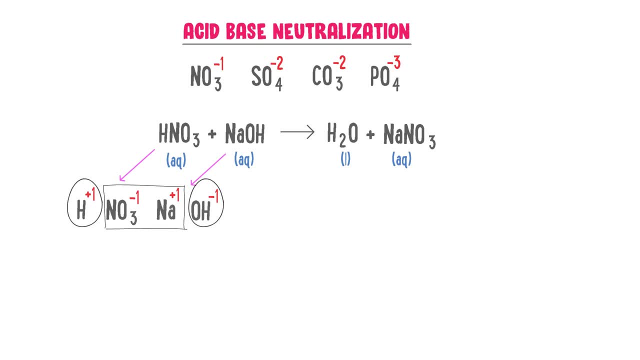 of sodium nitrate. Now let me balance this chemical equation. At this side of chemical reaction there is one hydrogen ion, one nitrate ion and one sodium ion and one hydroxide ion, While at this side of chemical reaction there is also one hydrogen ion, one nitrate. 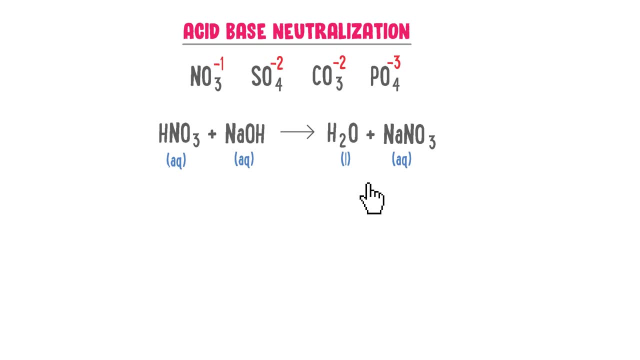 ion, one sodium ion and one hydroxide ion. So it is already balanced chemical equation. Secondly, I will write the net ionic equation. I write hydrogen ion plus nitrate ion plus sodium ion plus hydroxide ion. while at this, 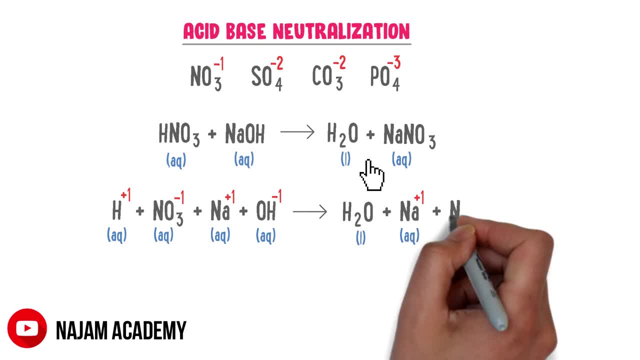 side: water and sodium ion plus nitrate ion. Remember that HNO3, sodium hydroxide and sodium nitrate are an aqueous solution. That's why I split their respective ions. Now cut the similar ions at both the sides, I get hydrogen ion plus hydroxide ion react. 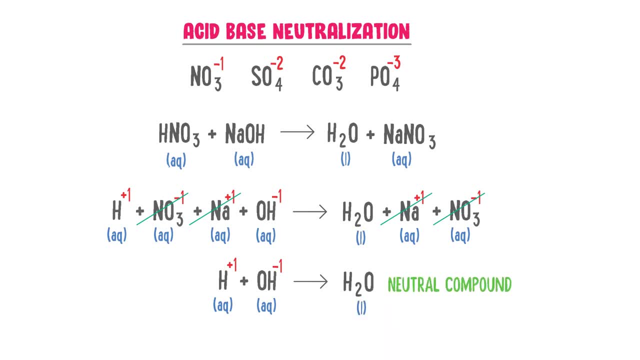 together to form water, And water is a neutral compound. We know that this hydrogen ion belongs to acid and this hydroxide ion belongs to base, So positive ion and negative ion neutralize each other to form a neutral compound called water. Therefore, this reaction of acid and sodium nitrate react together and form a neutral 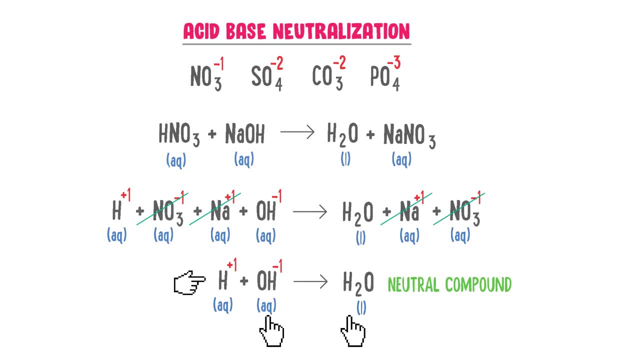 compound called water. Therefore this reaction of acid and sodium nitrate react together. Therefore, this reaction of acid and calcium nitrate react together and form a neutral compound called water. And here acid and base is called neutralization reaction, because positive and negative ion neutralize each other. Thus note it down, this neutralization. 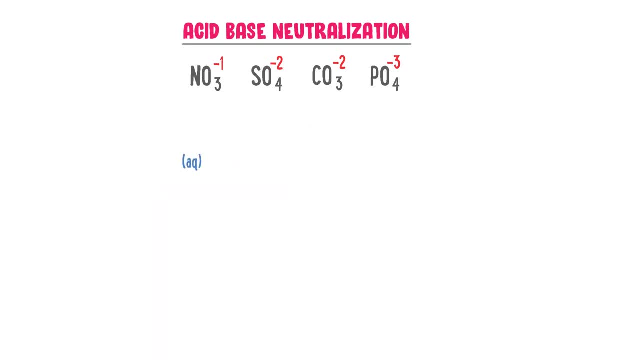 reaction. secondly, consider aqueous solution of acid like H2SO4 and aqueous solution of base like lithium hydrooxide. H2SO4 dissociates into hydrogen ion and sulfate ion, while lithium hydroxide dissociates into lithium ion and hydroxide ion. The positive hydrogen ion of acid react with the negative. 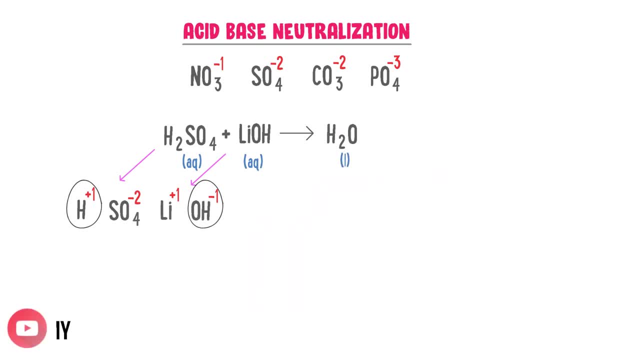 hydroxide ion of base to form water. Now how can sulphate ion react with lithium ion? Well, here write the sulphate ion, and we know it has negative 2 charge. And write the lithium ion here, We know that it has positive 1 charge. Now exchange the charges between them. So the chemical formula. 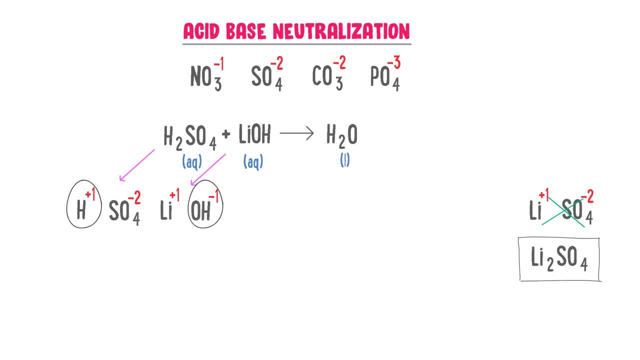 is lithium, 2 sulphate ion, Thus I write lithium, sulphate. Secondly, I need to balance this chemical equation. At this side of chemical reaction, there are 2 hydrogen ions, 1 sulphate ion, 1 lithium ion and 1 hydroxide ion, While at this side, while there is only 1 ion of hydrogen, 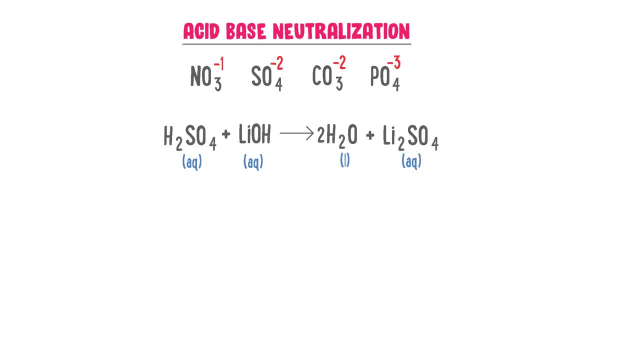 so I multiply it by 2.. Also, there is 1 sulphate ion While there are 2 ions of lithium. so multiply it by 2. and at both sides there are 2 ions of hydroxide. So this is balanced chemical reaction. Now let me write the net ionic equation. 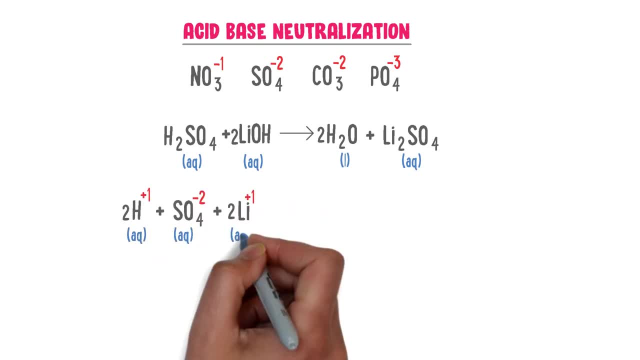 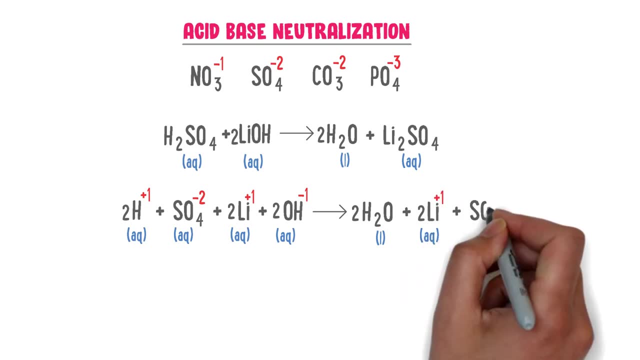 2 hydrogen ion plus 1 sulphate ion plus 2 lithium ion plus 2 hydroxide ion And at this side, 2 water molecule, 2 lithium ion, 1 sulphate ion. Now the common ions at both sides are: 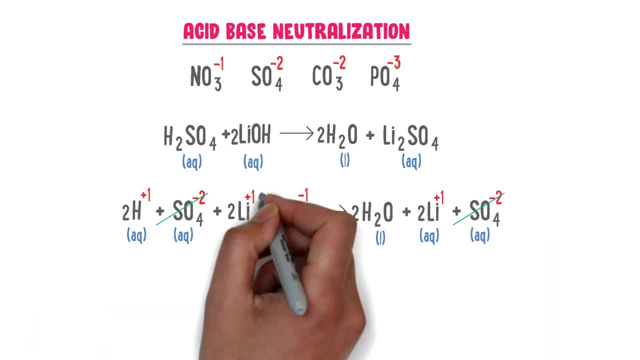 spectator ions And I cut these spectator ions at both the side, I get 2 hydrogen ion plus plus 2 hydroxide ion. react to form 2 molecules of water. I can divide both sides by 2 and I get hydrogen ion plus hydroxide ion to form water molecule. This is the net ionic equation, Hence noted down. 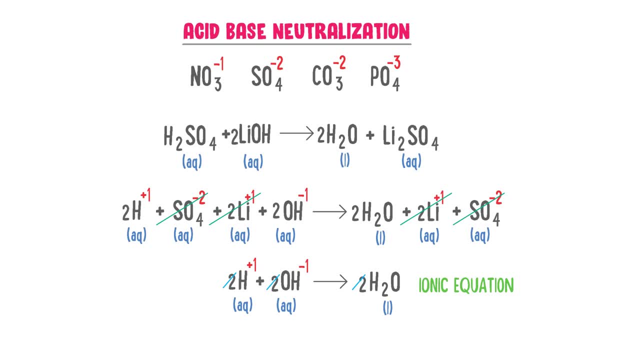 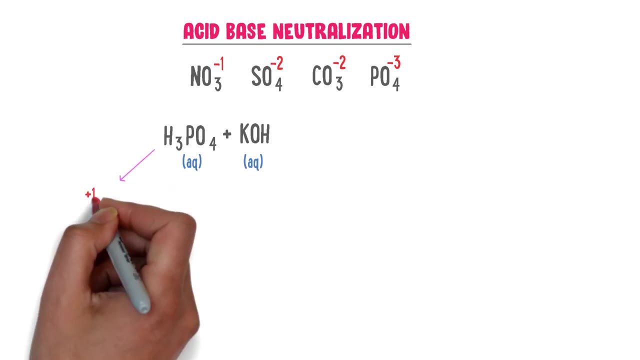 this neutralization reaction. Consider one another: acid base neutralization reaction. Consider aqueous solution of acid like phosphoric acid, and aqueous solution of base like potassium hydroxide. Phosphoric acid dissociates into hydrogen ion and phosphate ion, While potassium hydroxide dissociates into potassium.